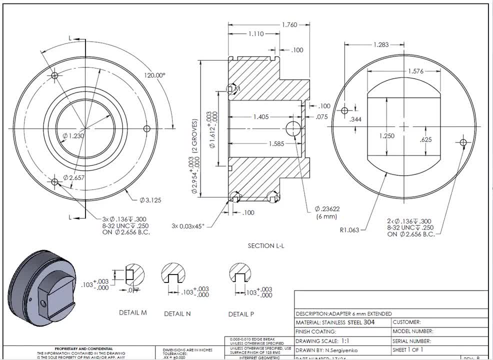 what kind of part was that? and figure out all the missing dimensions. Let me explain it on an example. Let's say you don't have this dimension but you need it. okay, you desperately need it for your calculations. So let's say: you don't have this dimension but you need it- okay, you desperately need it for your calculations. so 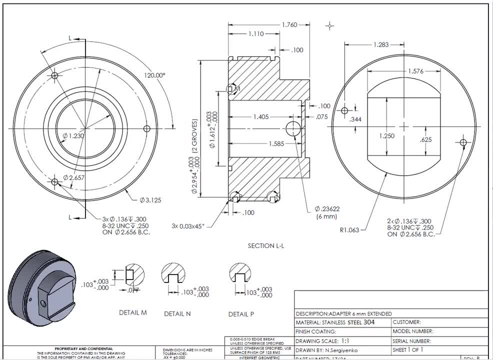 what you do? you have overall dimensions, which is 1.760, and you have this part, which is 1.110. so what you do is just do simple calculations. you take a whole length: 1.1 and 760, I'm sorry, minus 1.110. so whatever you got is: 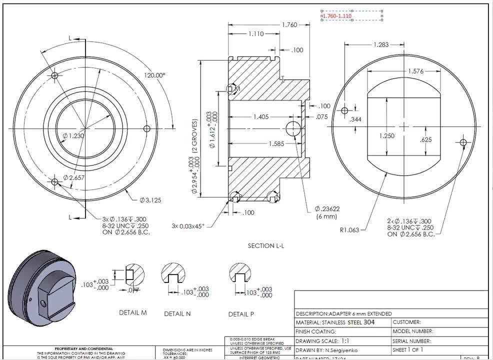 will be your missing dimensions. all the rest story was all the rest dimensions. so drawing will provide you not all the information, but enough to calculate whatever you need. okay, okay, let's go a little bit closer to the top view. so this is a- I'm sorry, this actually the. 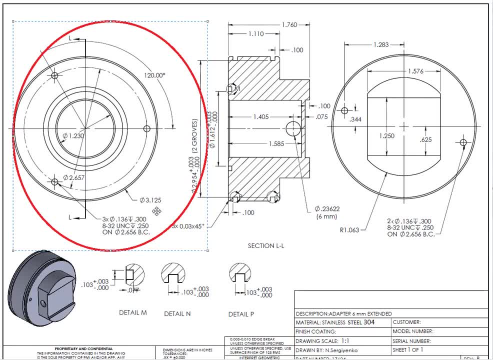 bottom view. so it gives you information how big this circle, okay, how big this part. so this is the overall diameter. so this, this symbol on a tap, it means diameter. you can also do with the radius. radius it's like this R and whatever is that. you know, diameter is twice bigger than radius. 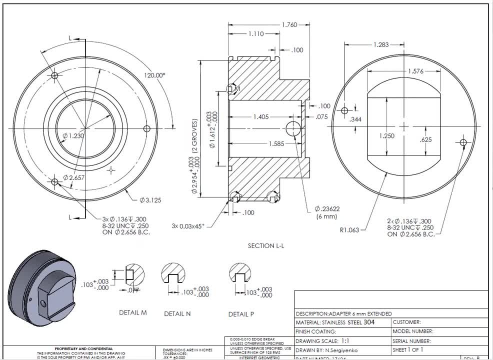 It gives you some other dimensions, and let's look this one. it's very tricky and very interesting. so you will tap three holes in the bottom of the part. so it says we have three holes. it gives us diameter of those holes and how deep they go. if you notice all the, everything goes in a thousandth of an inch, even if it. 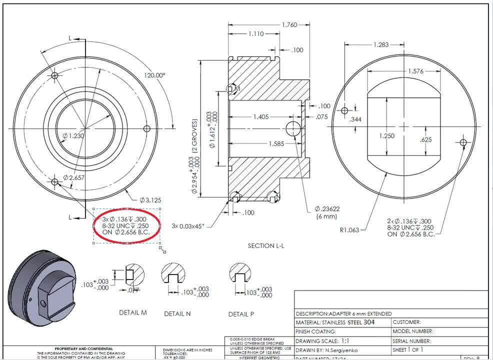 says three hundred thousandth of an inch, we don't run. just point three. reason why is because machine shop works in a thousandth of an inch. it's a unit, how much in shop works okay. so if you go on second line that says 832, 832, it means 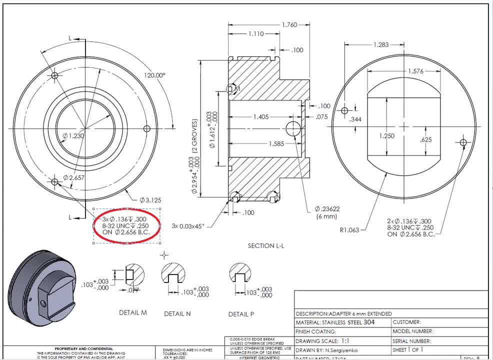 what kind of thread is that? UNC thread? and it goes two hundred and fifty thousand inch deep. we don't say core range, we say two hundred and fifty thousand inch deep. and third line gives us information about location of those holes. so what does it mean? on diameter, two point six, five, six BC. BC means both. 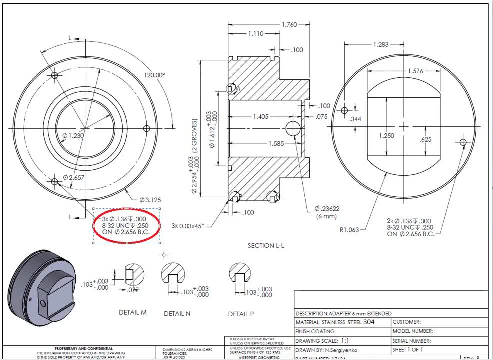 circle, Both circles, imaginary circle, where all those holes located evenly spread it. so in our case we have three holes, so 360 degrees. we divide by three, so we have 120. so that's what gives us here. okay, so we have. now we have idea what kind of. 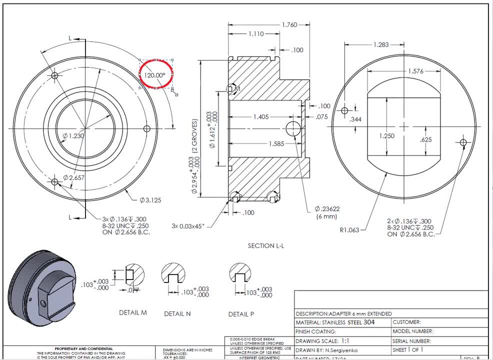 holes, how deep they are, how deep they are and where they are located. okay, the same story over here is holes on the top. it's how it works. okay, this part means it's a chamfer. it means we have three chambers on this part. well, we don't want to have any sharp edges. we don't want. 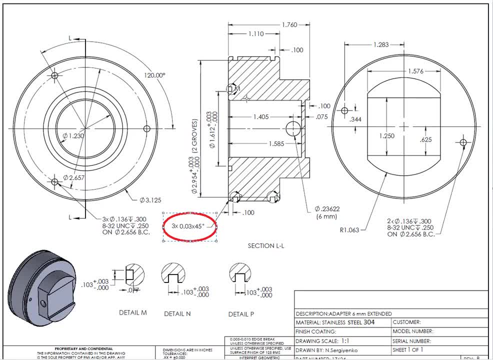 anybody to get hurt. so we give some information about those sharp edges. this is one, this is two and this is three over here. okay, that's what we have, and you also see those little things. it's very, very small space. it's not enough to provide all the necessary. 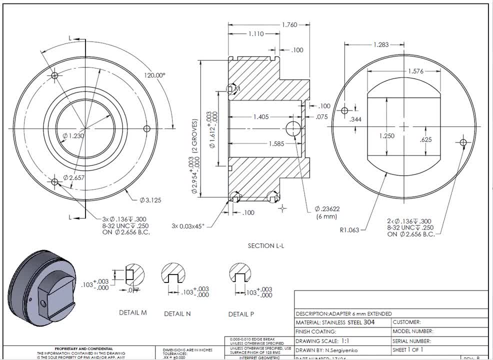 information. so what we do? we have detail of use M and MP, so it gives information about your o-ring grooves, okay. 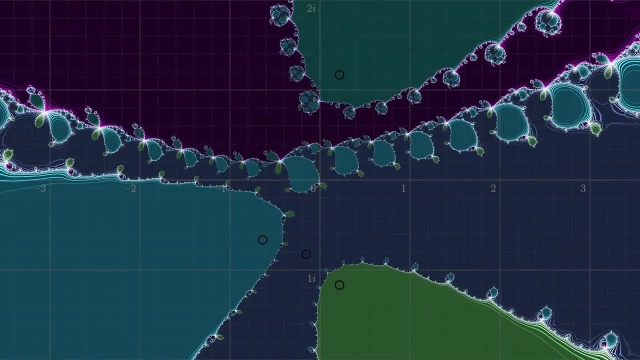 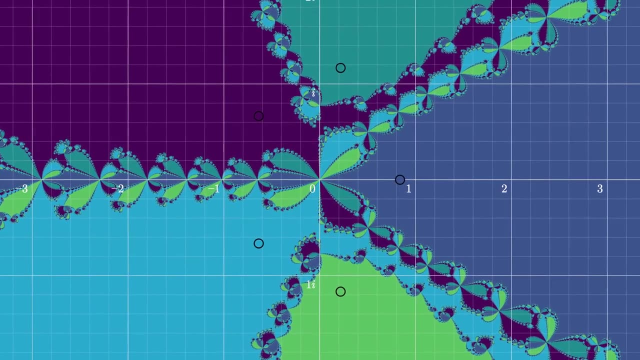 You've seen the title, so you know this is leading to a certain fractal and actually it's an infinite family of fractals And, yeah, it'll be one of those mind-bogglingly intricate shapes that has infinite detail, no matter how far you zoom in. But this is not really. 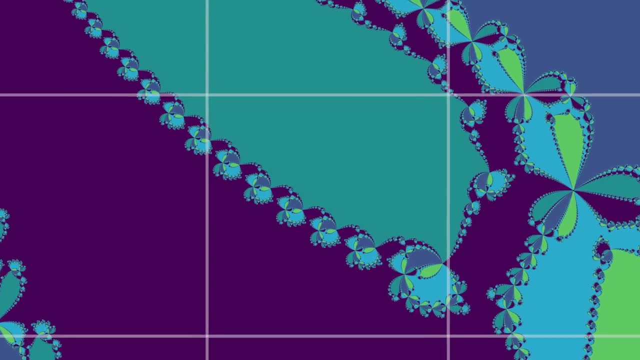 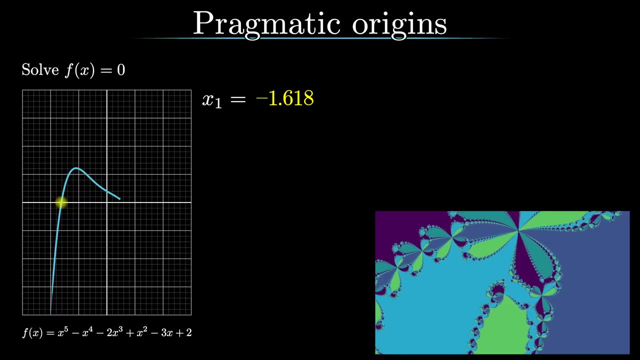 a video about generating some pretty picture for us to gawk at. Well, okay, maybe that's part of it, but the real story here has a much more pragmatic starting point than the story behind a lot of other fractals And, more than that, the final images that we get.